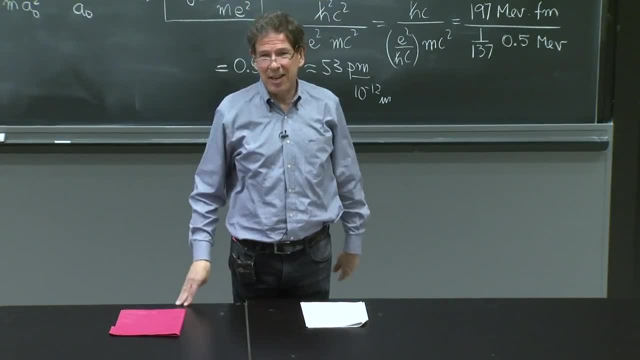 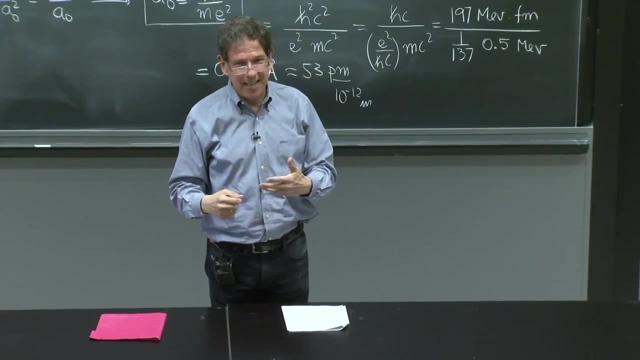 But here you get the energy levels, and you get the exact energy levels. So it's a nice thing that in quantum mechanics, energy levels are things that you calculate exactly. Of course, when you try to measure energy levels experimentally, the uncertainties arise again. 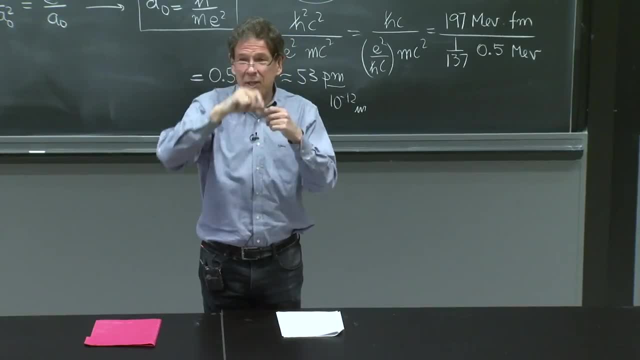 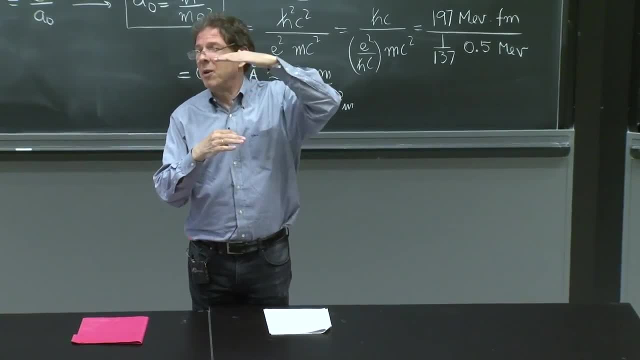 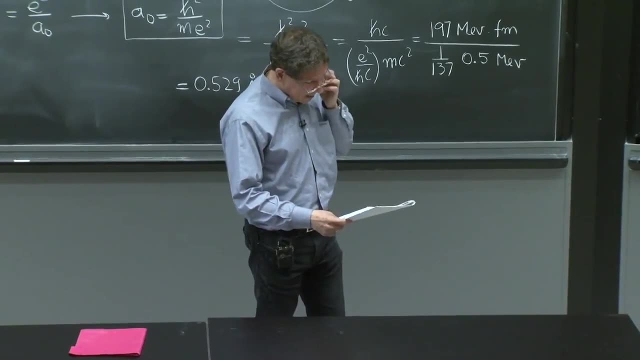 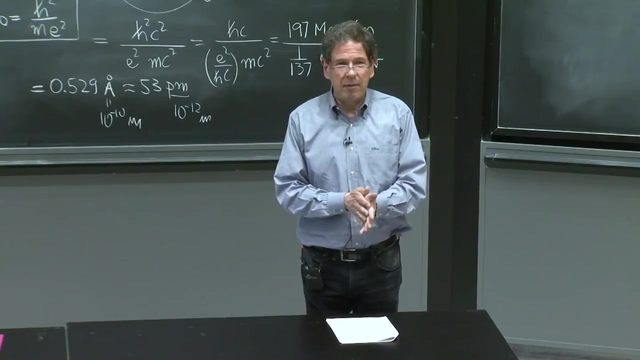 But the end result is that these systems have beautifully determined fixed numbers called energy levels, And that's what we're aiming at. It's a nice thing because it's the most physical example. It has many applications: the energy levels of hydrogen atom. 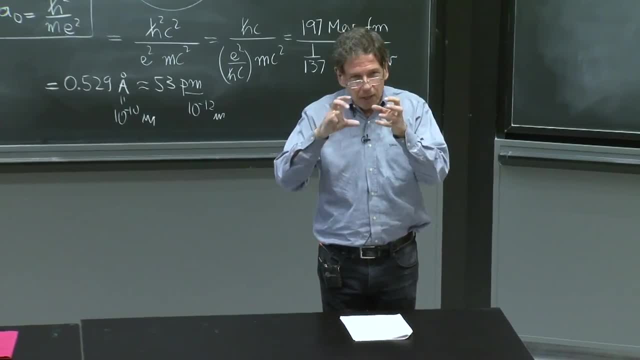 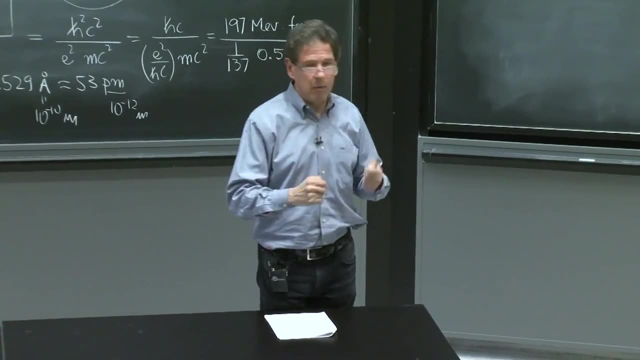 The more you study, the more complicated they are, because you can include fine effects like the effects of the hydrogen atom, The effects of the spins of the particles- what does it do? The effects of relativity- what does it do? 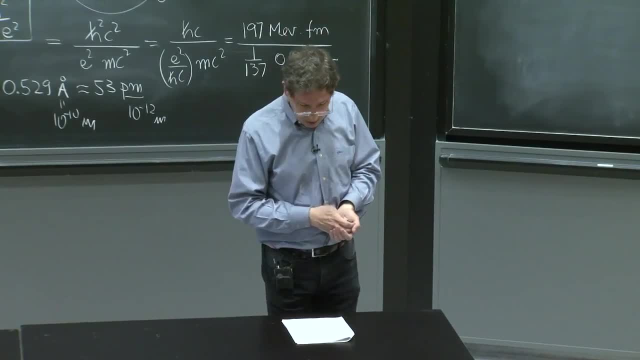 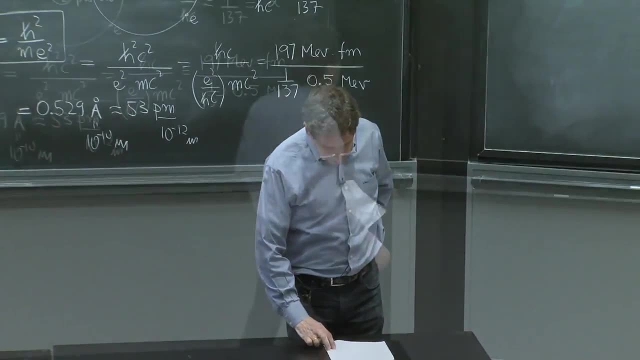 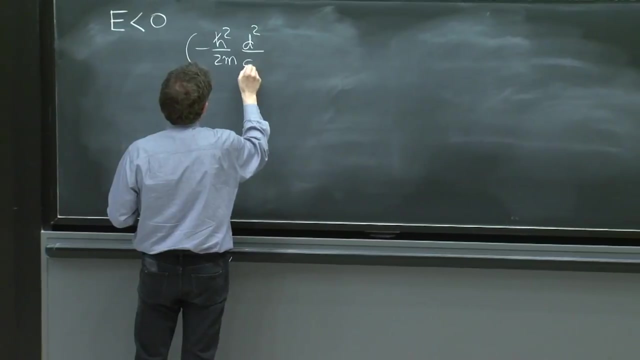 All kinds of things you can put in and do more and more accurate results. So it's really unbelievable how much you can learn with the fine spectrum of the hydrogen atom. Our equation is: minus h squared over 2m d, second dr squared, the radial equation. 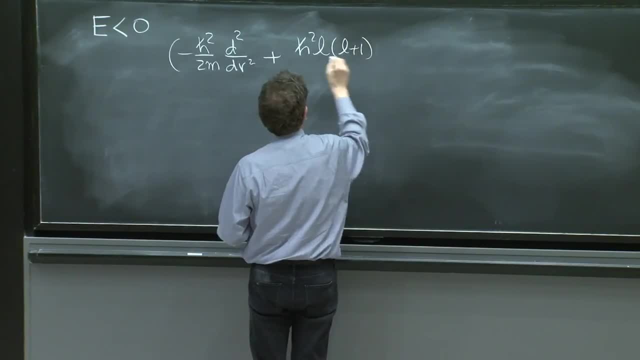 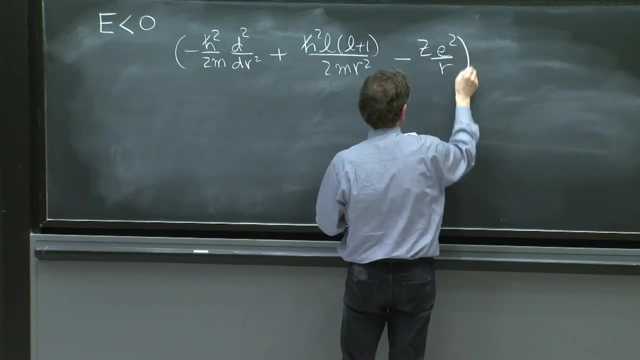 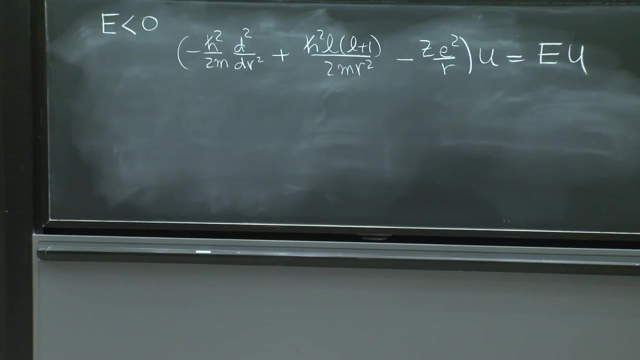 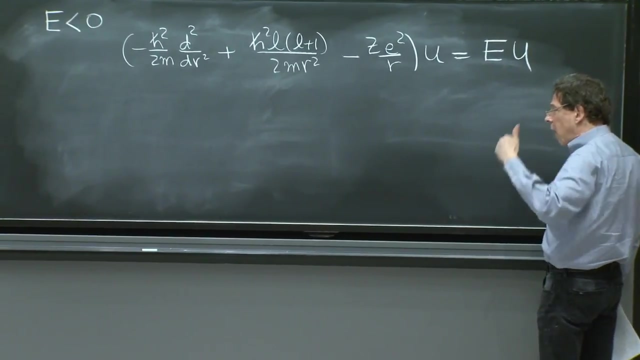 L times l plus 1 over 2m r squared minus z e squared over r, u is equal to eu. So this is the radial equation. Remember it was like a Schrodinger equation for a variable u And the wave function was u over r times a psi, lm or a ylm. 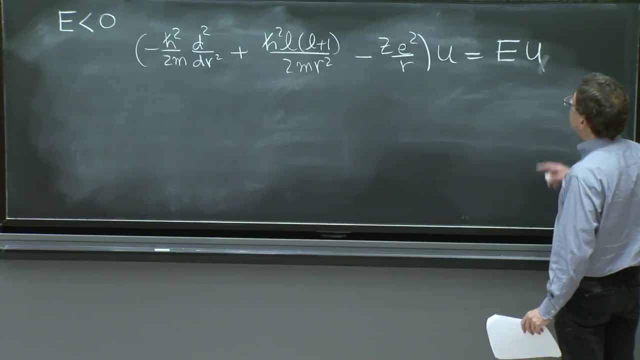 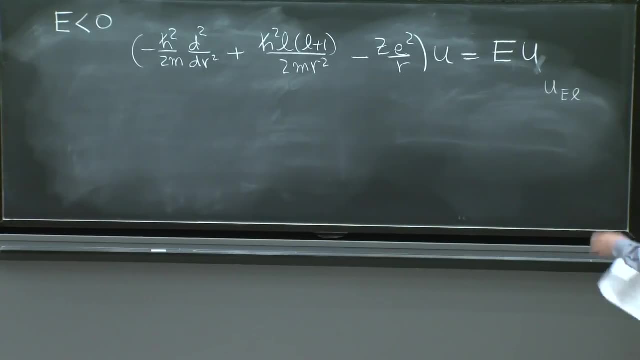 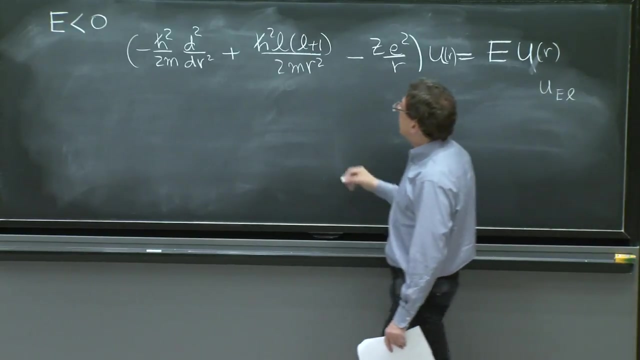 actually It's a spherical harmonic. Here I could have labeled u with e and l, because certainly u is u of r And u depends on the energy that we're going to get And it will depend on l that is there in the differential equation. 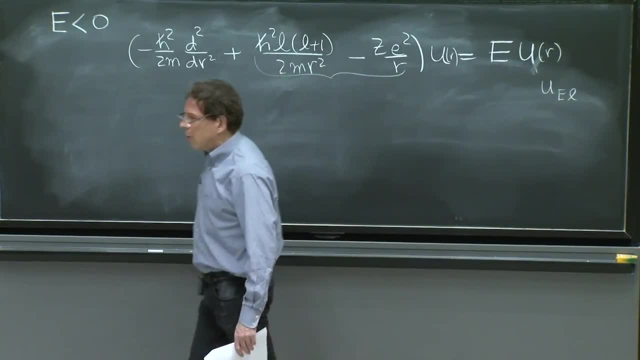 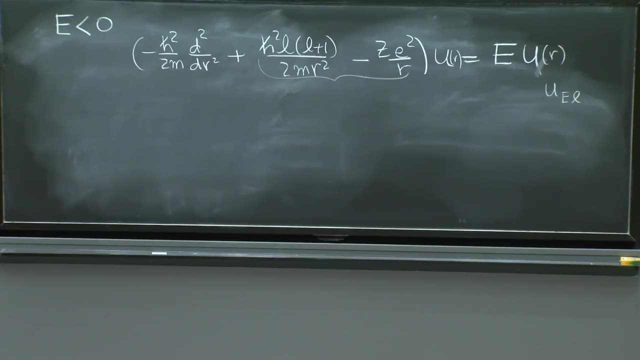 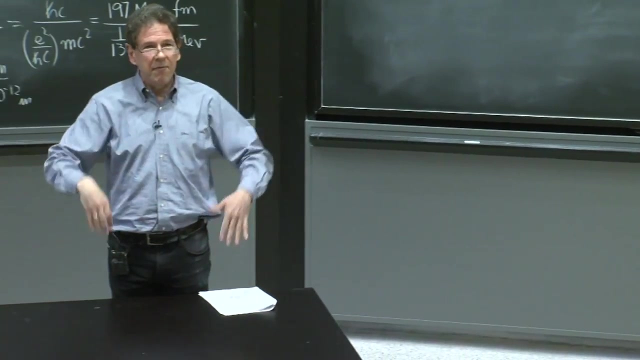 This is the effective potential that we discussed before. It was the original potential, To which you add the centrifugal barrier. And what are you supposed to solve here? You're supposed to solve for l equals 0, to find some states for l equal 1,, 2,, 3,, 4, infinity. 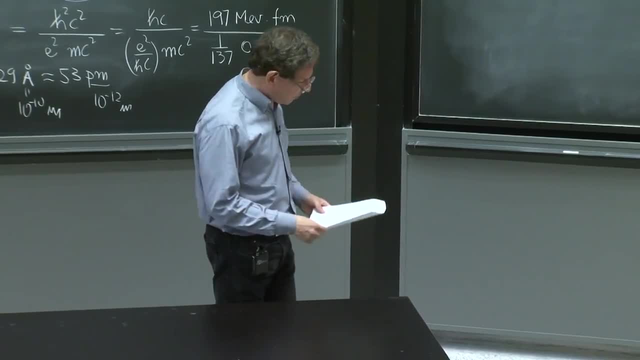 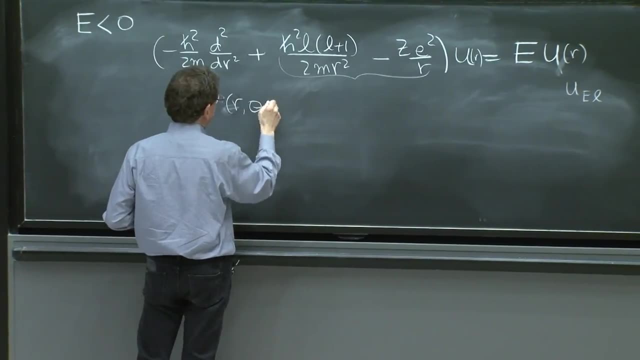 You should find all the energy levels of this thing. So the wave function is psi of r theta, and phi will be this: u of r over r times a ylm. So it's going to be u of r over r times a ylm. 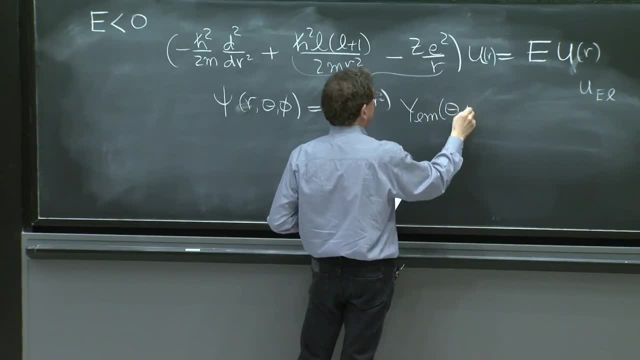 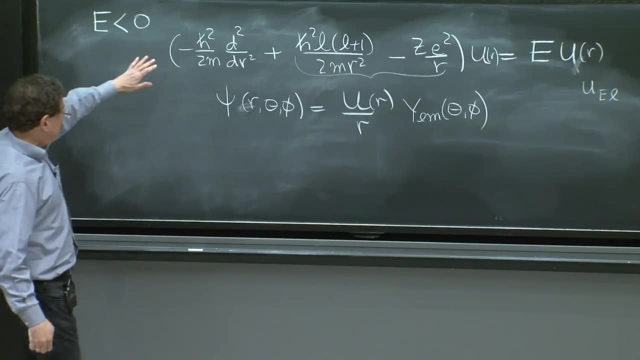 So it's going to be u of r over r times, a ylm of theta and phi, And in fact plugging that into the Schrodinger equation was what gave us this radial equation. So this was called the radial equation which we talked about. 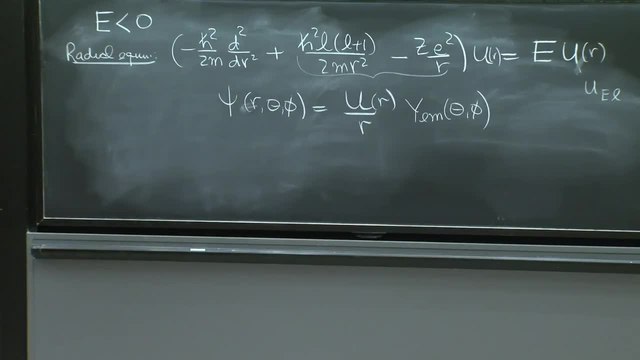 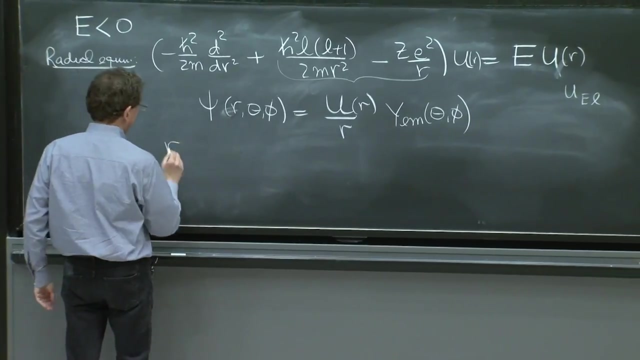 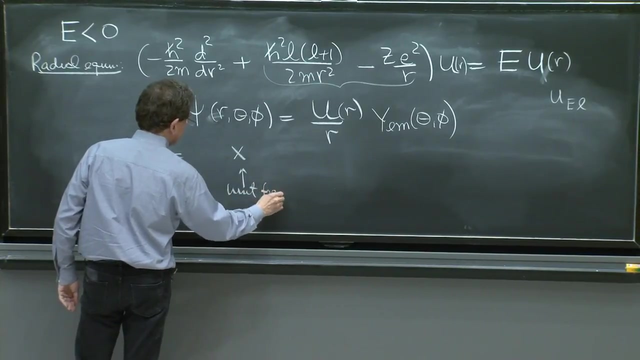 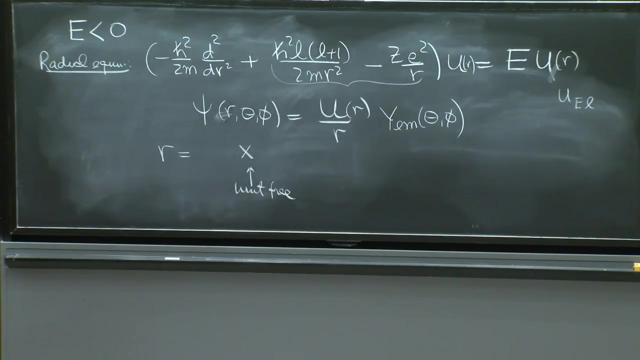 We never quite solved it for any particular example. As you know, we like in this course to get rid of units and constants, So first. So now, the first step is to replace Our by a unit free, x, x, And we have the right quantity, a zero. 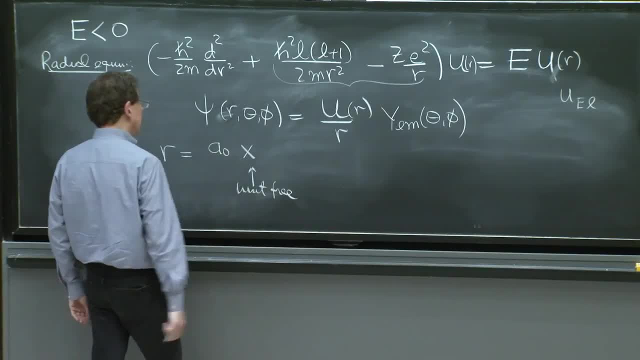 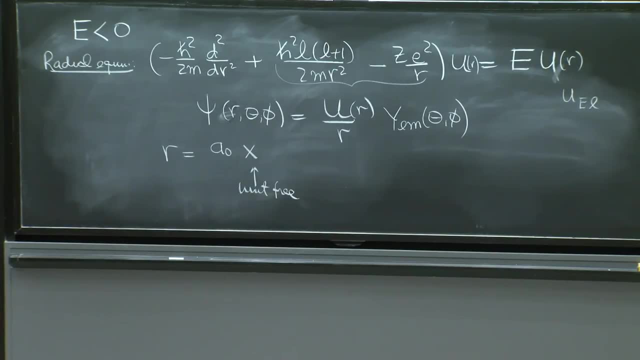 A zero would be the perfect thing. So if you do that, you will be able to clean up the units. But But If you, you might not quite be able to clean up. 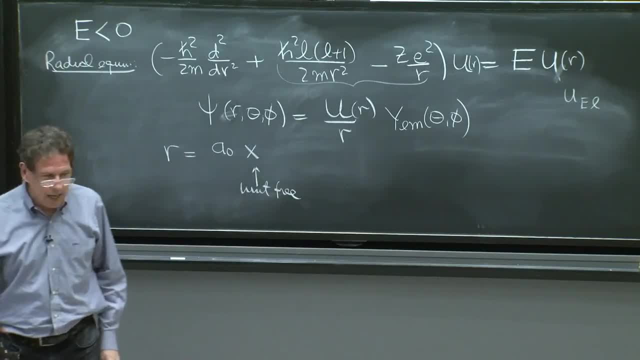 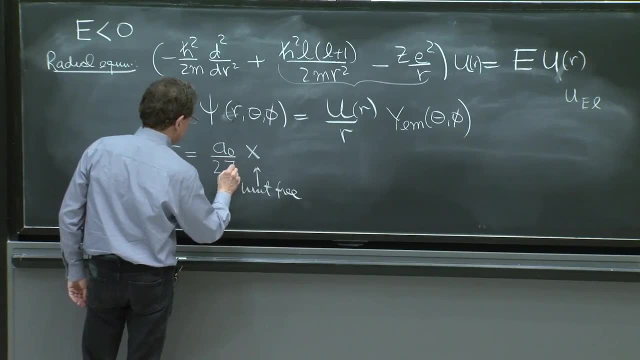 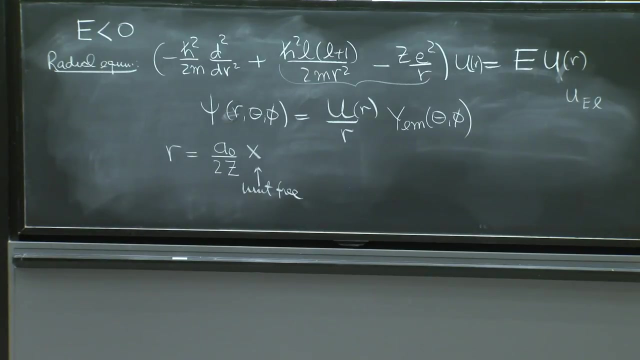 the z from all the places that you would like to clean it up. So we can improve that. Maybe it's not too obvious by putting a 2 over z here. z has no units, of course, So that you would probably do by trial and error. 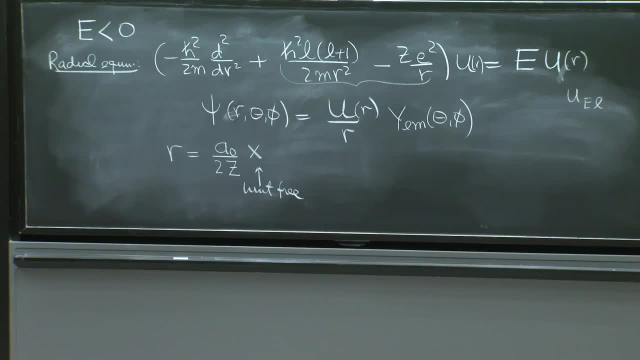 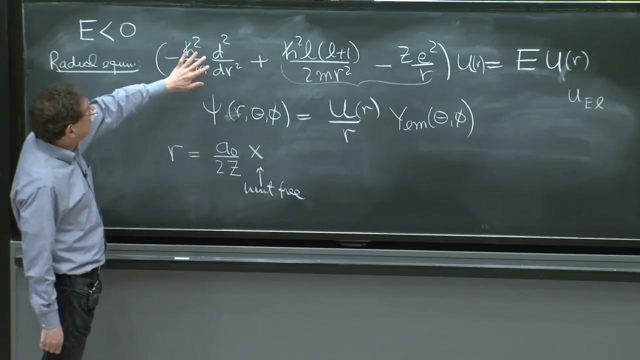 You would say: well, I want to get rid of the z as well, And I have it in this form And you will see how it works out. So at this moment I have to plug r into this equation and just clean it up. 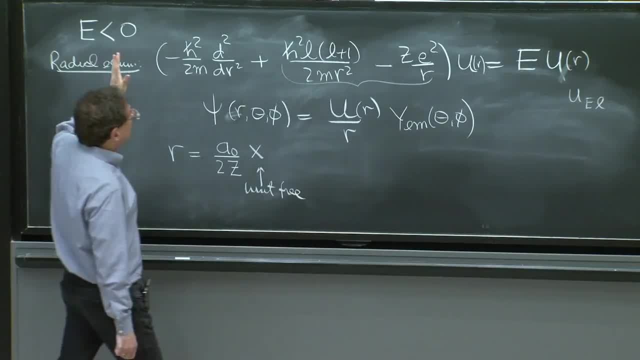 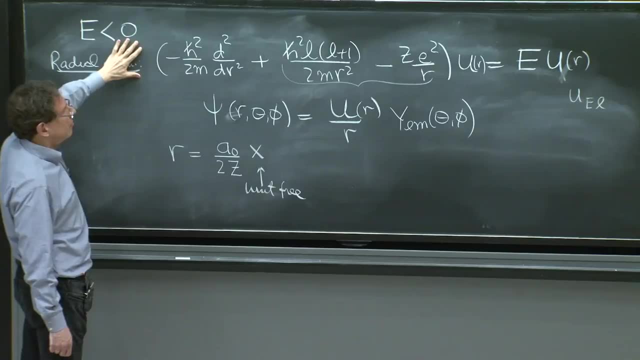 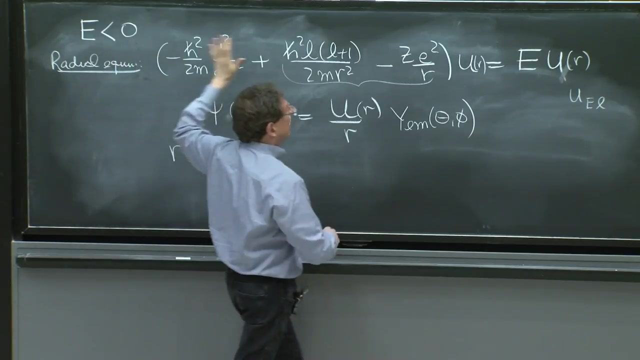 And what should happen is that everything, all the units, should give you A factor with units of energy, Because, at the end of the day, if whatever is left is not going to have units, everything out must have units of energy. So this takes about one line to do. 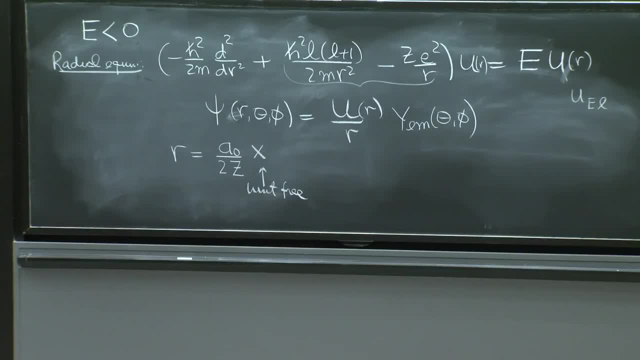 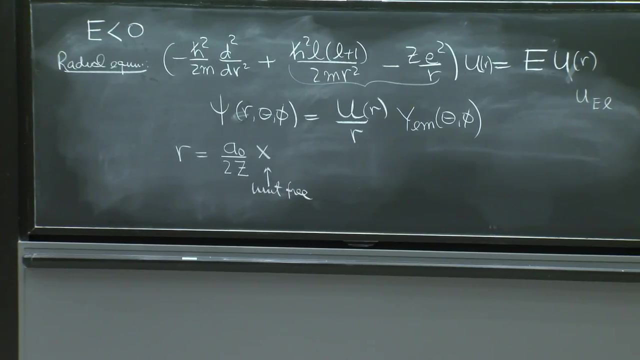 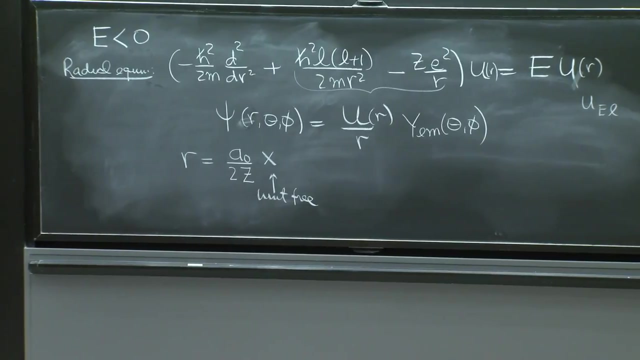 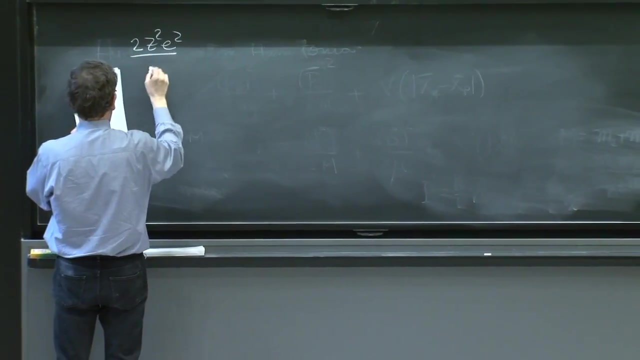 I'll skip some algebra on these things. I'll try to post notes soon on this. So if you leave a line, You could do the calculation for yourselves And it might be worth it. The claim is that we get 2z squared e squared over a0. 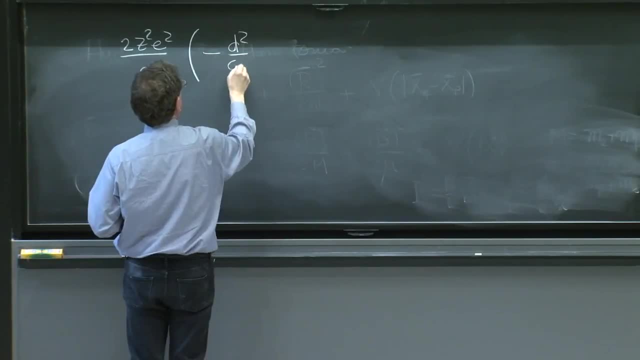 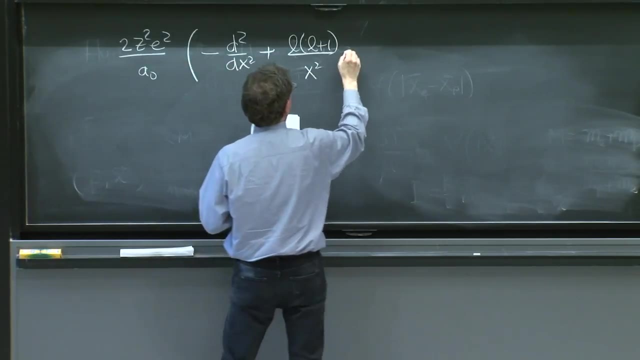 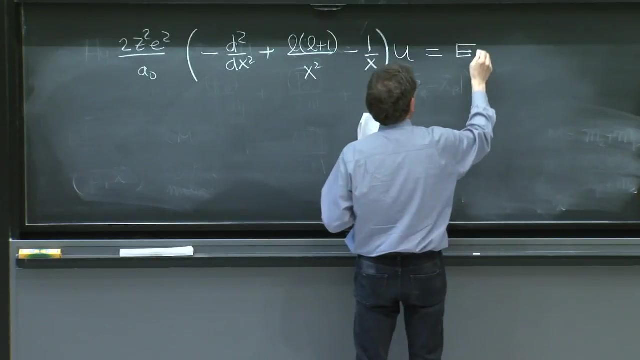 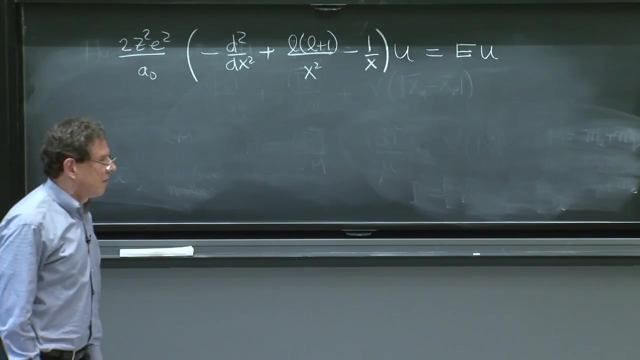 multiplying minus d. second dx squared plus l times l plus 1 over x squared. That's the claim. So we get 2z squared minus 1 over x times u equals eu. That will be the common factor that will come out of everything. 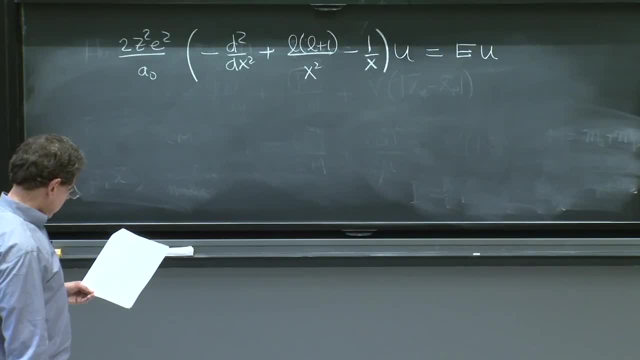 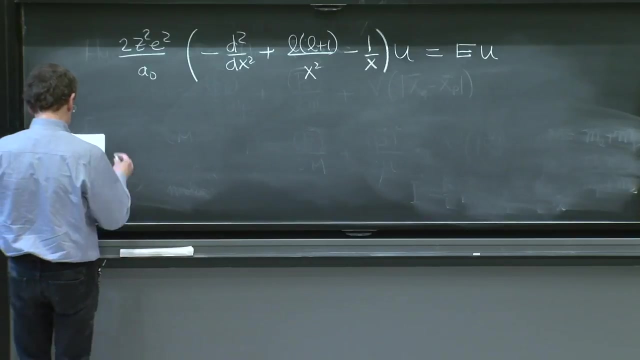 by the time you solve it, And it has the units of energy. as you can imagine, e, squared over a0, has the units of energy, So might as well move that to the other side to get the final form of the equation, which. 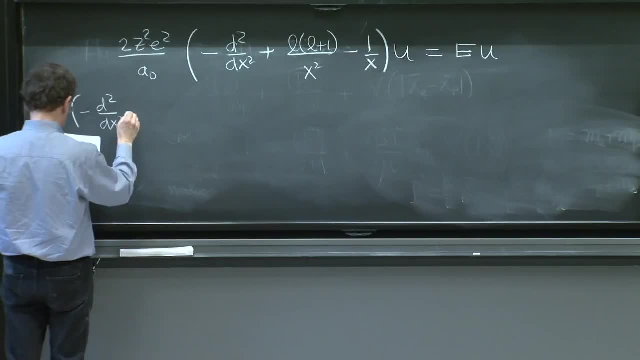 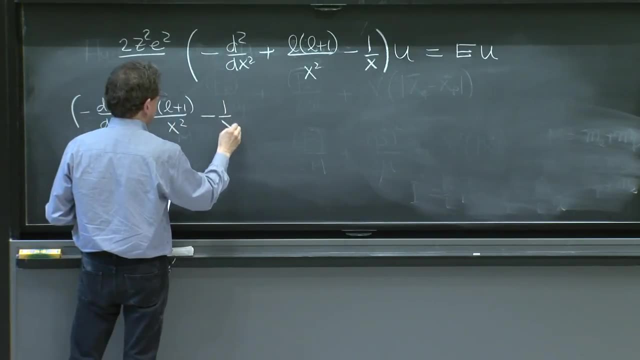 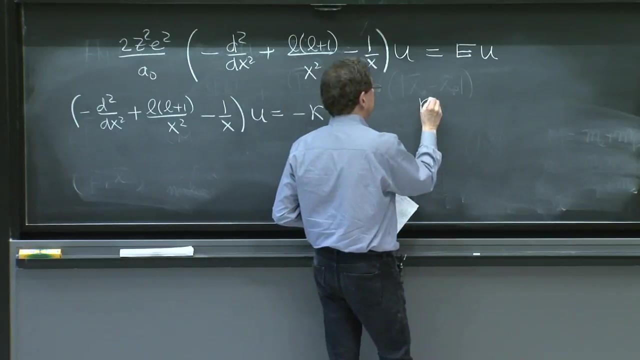 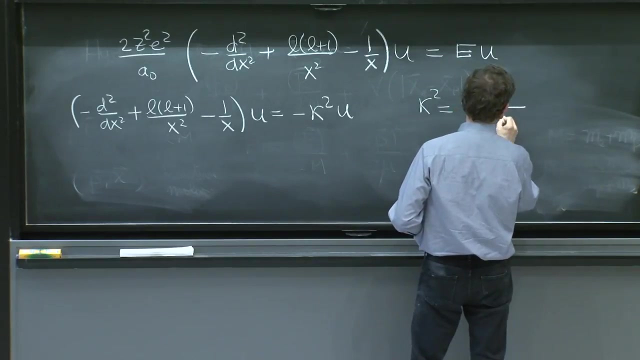 would be minus d second dx squared plus l times l plus 1 over x squared minus 1 over x? u is equal to minus kappa squared u, Where kappa squared is going to be minus e over 2z, squared little, e squared over a0.. 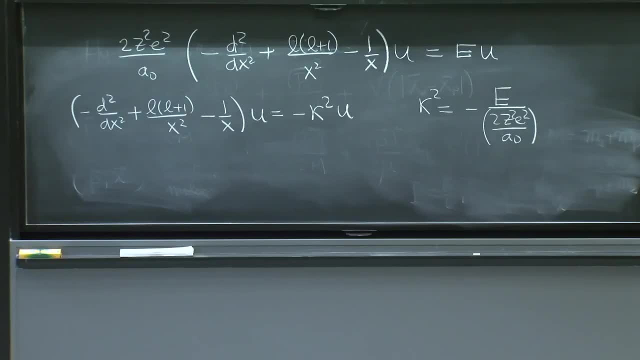 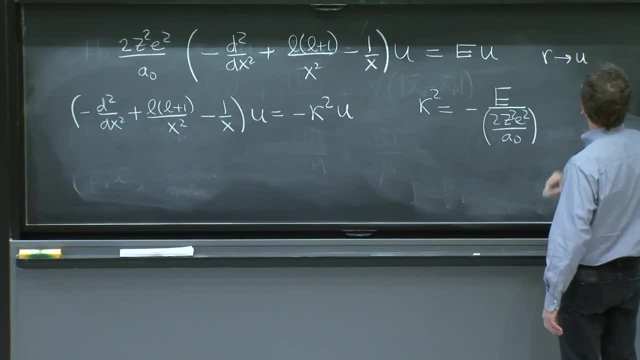 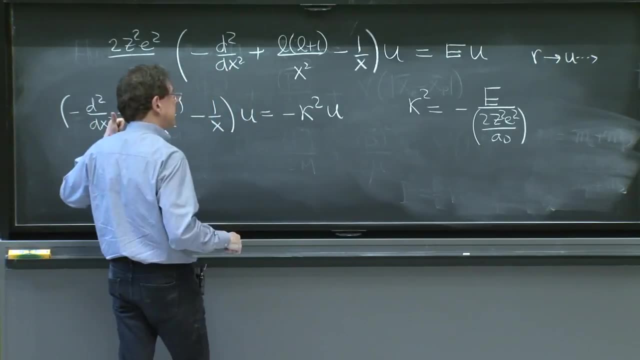 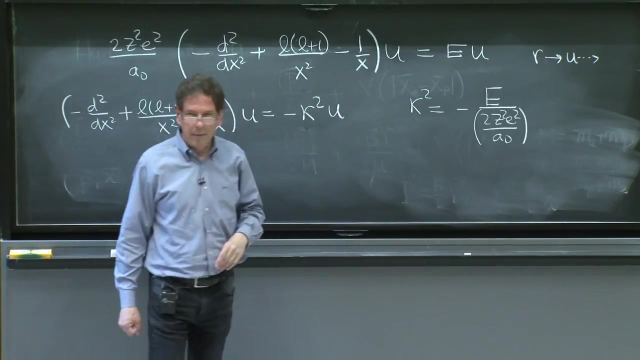 So let me just re-emphasize what's going on here. We've passed from r variables to u variables. We will still do more things, And we have a0 in there, z in there, And then the energy is really encapsulated. 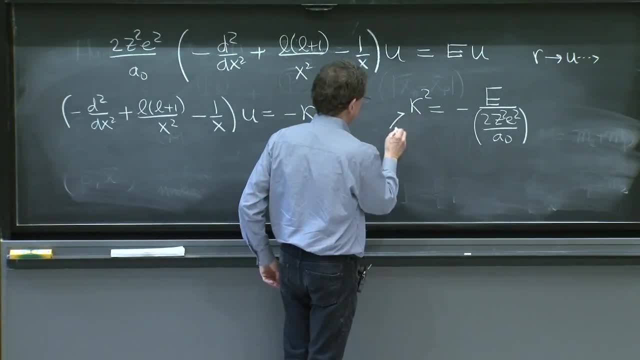 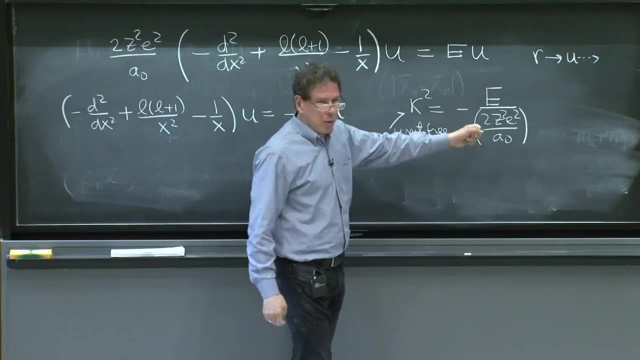 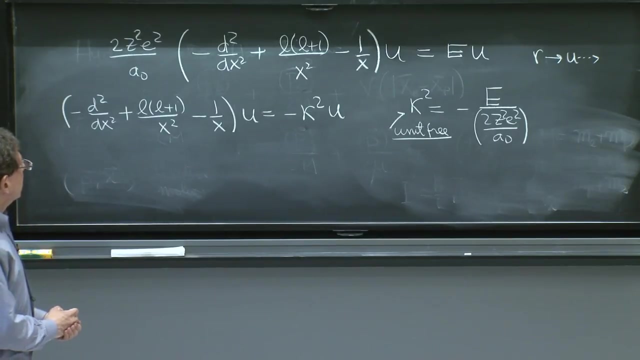 And it's kappa is unit-free. So if you know kappa, you know the energies. That's what you should be looking for. Kappa is the thing you want to figure out. Knowing kappa is the same as knowing the energies, because this is just a constant that gives you 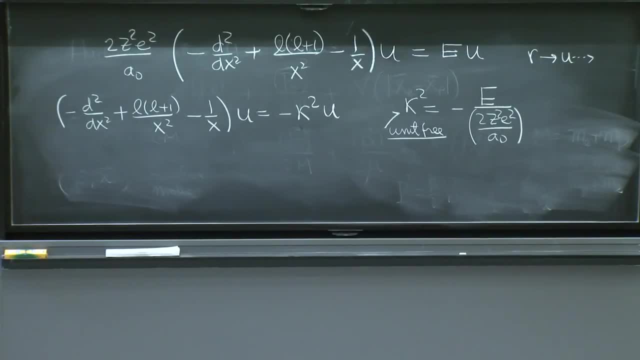 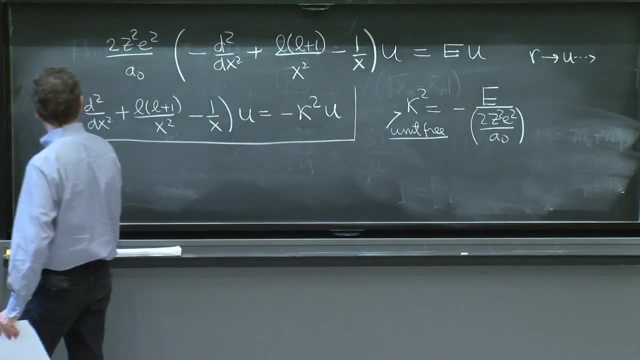 the scale of the energy. So this is what we want to solve, So, and the equation doesn't look all that complicated, but it's actually not yet that simple, unfortunately, So we have to keep working with it a bit. So one reason: you can see that an equation like that 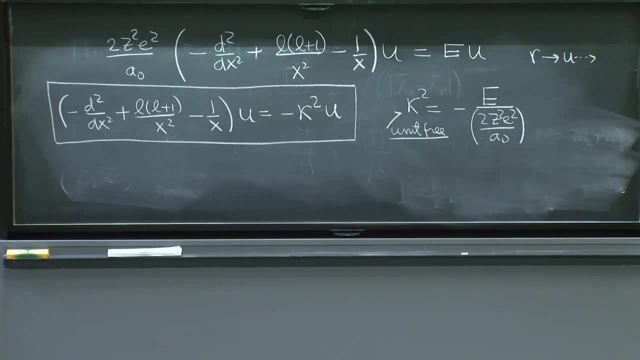 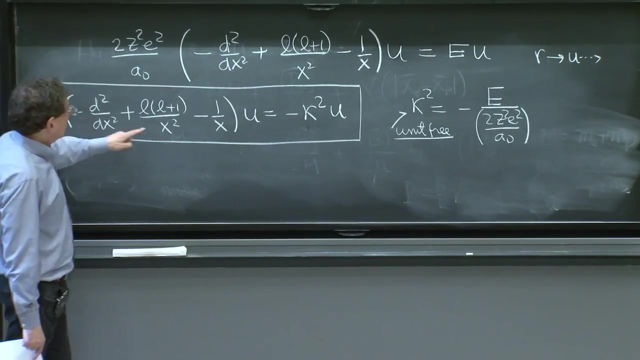 would not be too simple is to look at it and see what kind of recursion relation it would give you. And that's a good thing to look at at the beginning. And you see, OK, here I'm going to lower the number of powers. 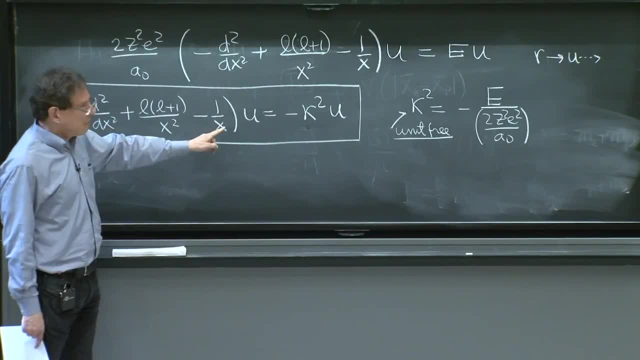 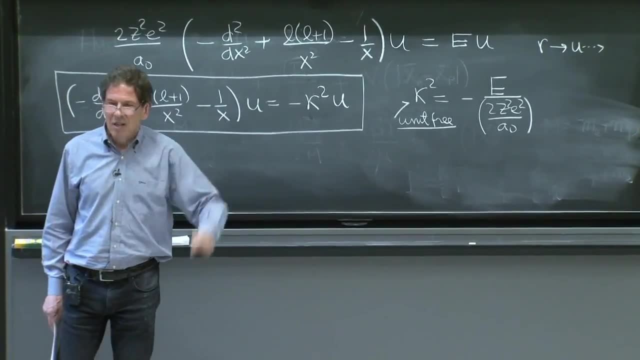 by 2.. Here I'm going to lower the number of powers by 1. And here I'm not going to lower the number of powers. So you're going to have three terms. So it's not a simple recursion relation which the next term is determined. 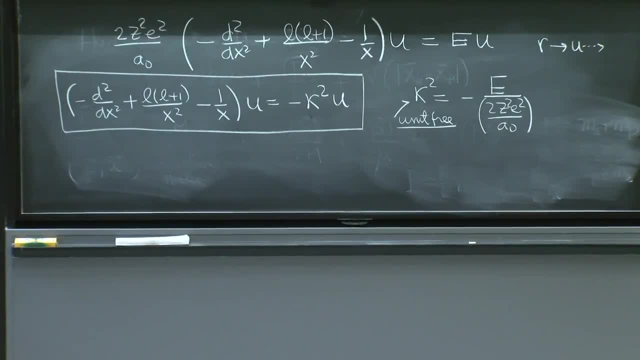 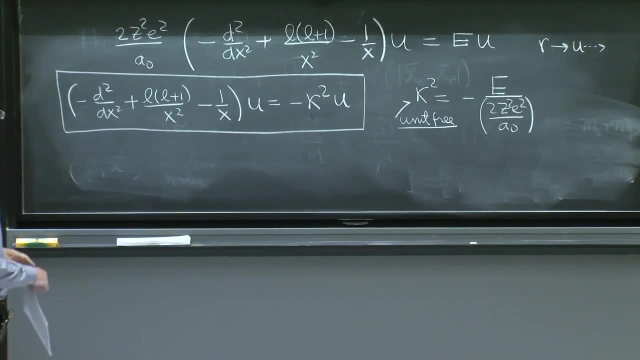 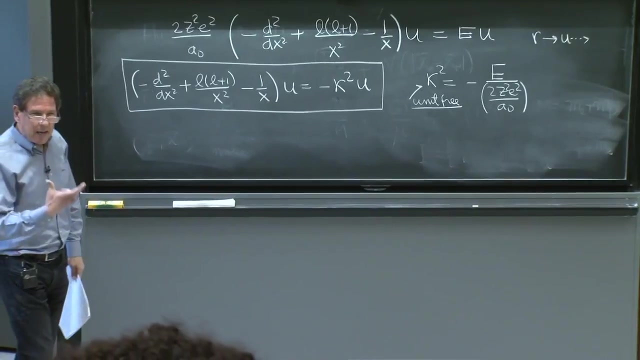 by the previous one. So that suggests you better do some work still with this equation. It's a good thing to simplify the situation And several things that you can do. One thing is to look at the behavior of the equation- near infinity, near 0, and see if you see patterns going on. 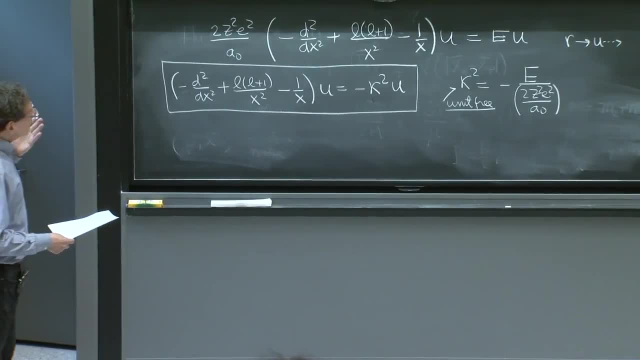 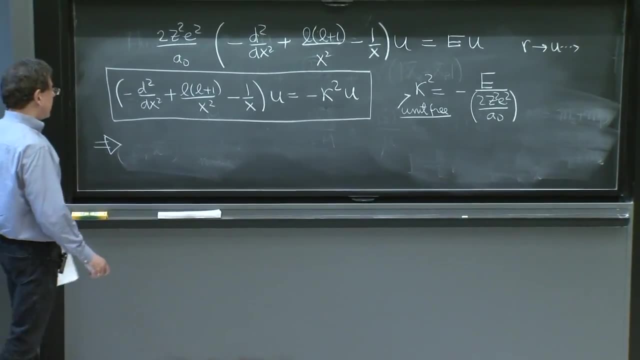 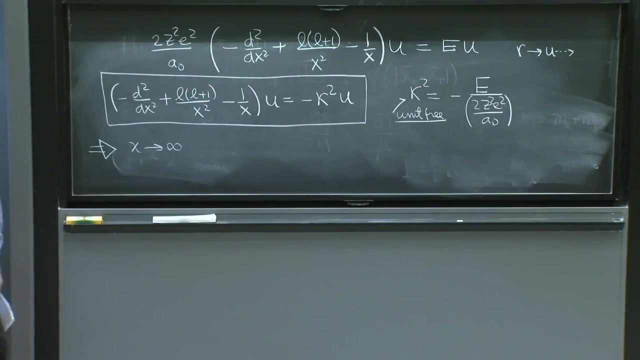 One thing we're going to do is to- which is not urgent, but it's usually done and people do it in different ways- is to look at x goes to infinity And see what the solutions may look like. So, as x goes to infinity, the differential equation probably. 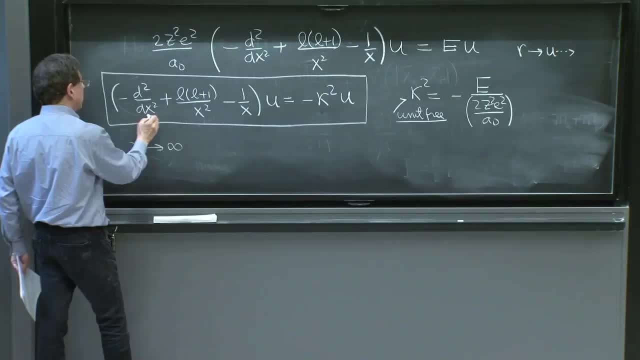 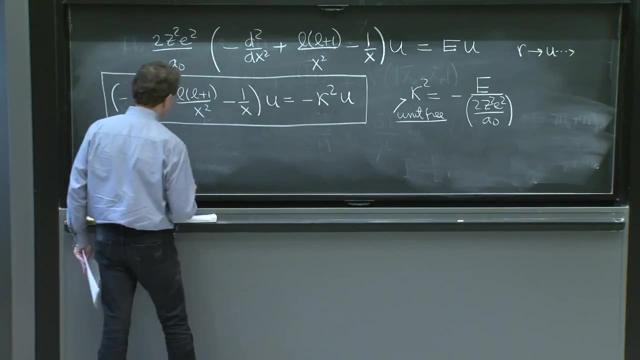 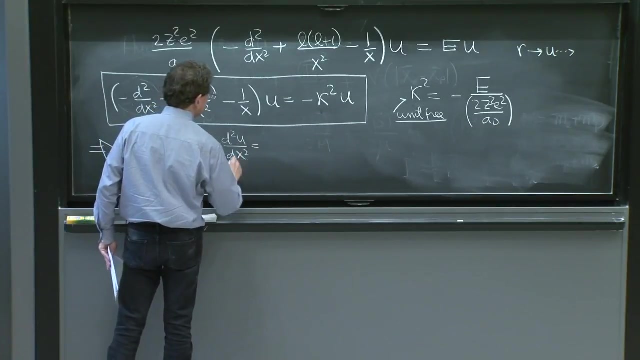 can be approximated to keep this term to see how things vary. And x goes to infinity. throw this, throw this and keep that, So you would have d second u: dx squared is equal to kappa squared. OK, OK, So that's the third. 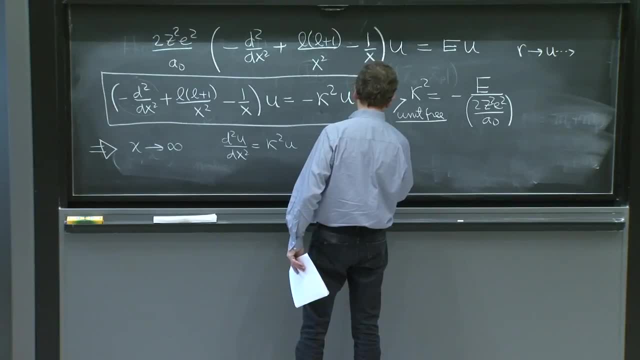 So this suggests that u goes like e to the plus minus kappa x, So exponential behavior: e to the plus minus kappa x. Ideally, of course, for our solutions we would like the minus 1, but we Now. this suggests yet another transformation that people do, which is: look, kappa is dimensionless. 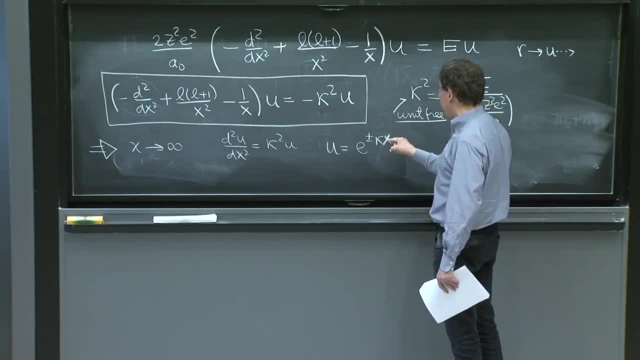 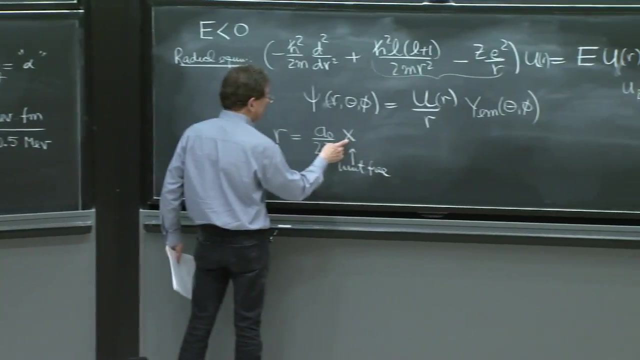 And we had x that is unit-free also. So kappa has no units, x has no units. So let's move to yet another variable. You see, we started with r being proportional to x, And now we can put factors that may help us without units here. 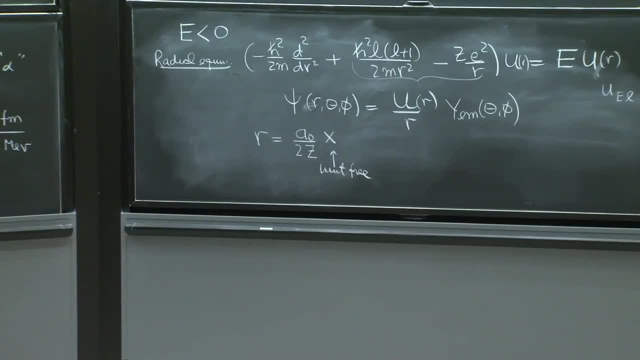 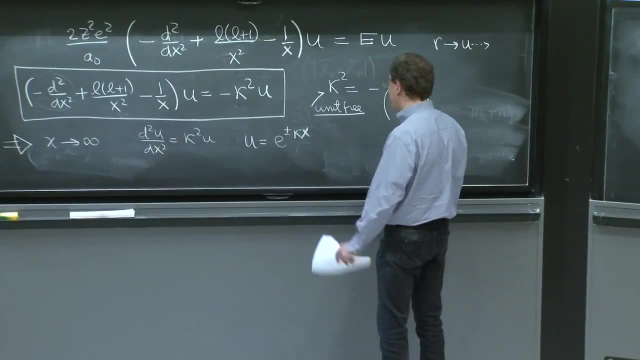 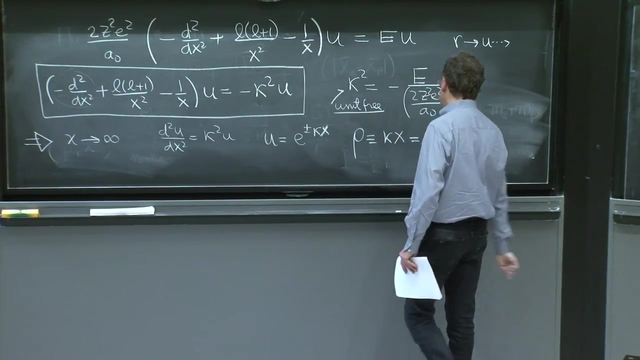 So I'm not suggesting that this is something that would occur to me if I'm doing this problem, But it's certainly a possible thing to do To say, OK, I'm going to define now rho as kappa x And with x being given by this rho. 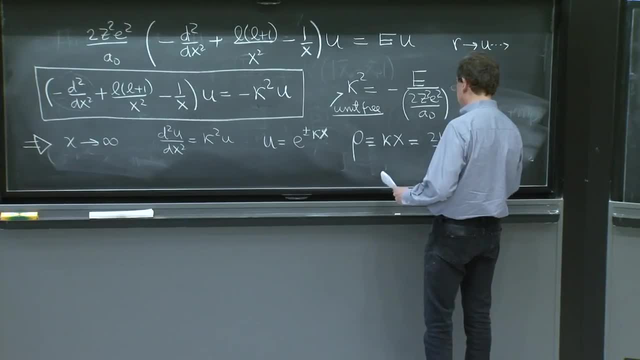 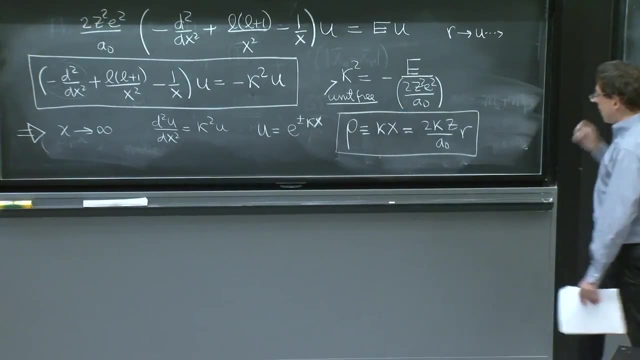 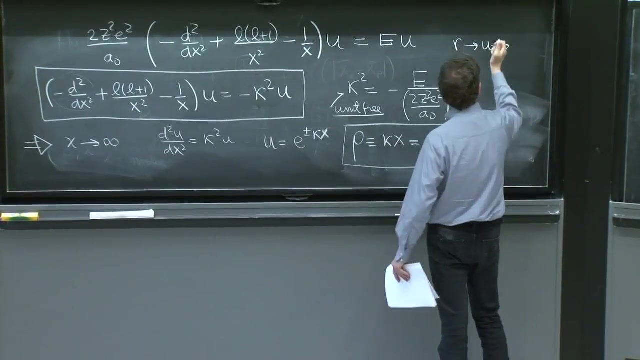 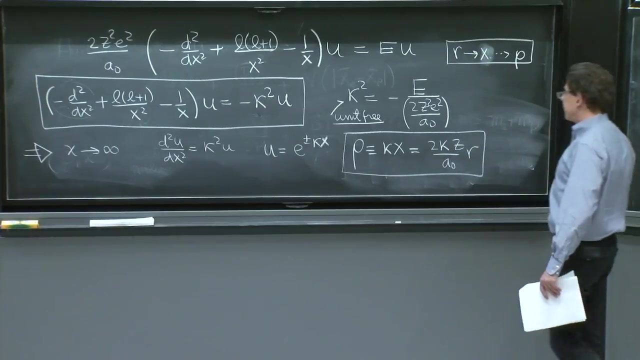 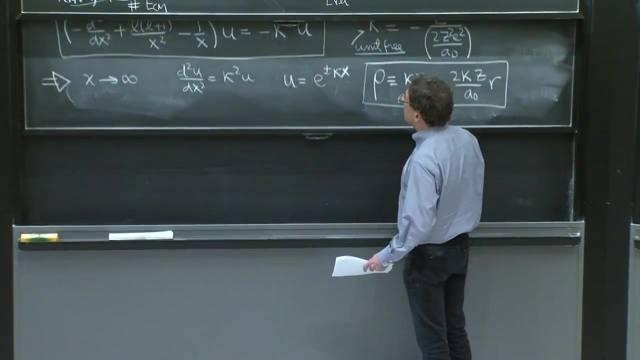 would be 2 kappa z over a0 r. So rho is going to be my new coordinate. So from r, I'm sorry- we've gone to x And now we've gone to rho, a new variable over here. So what happens to the differential equation? 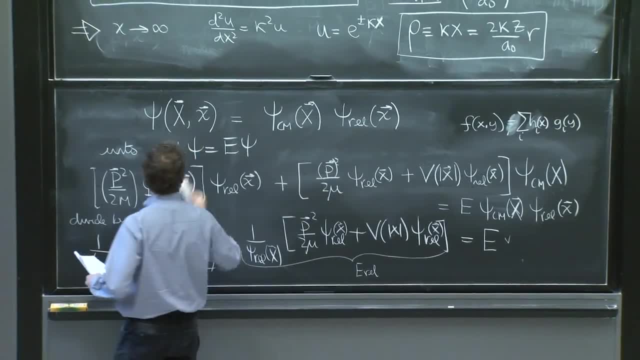 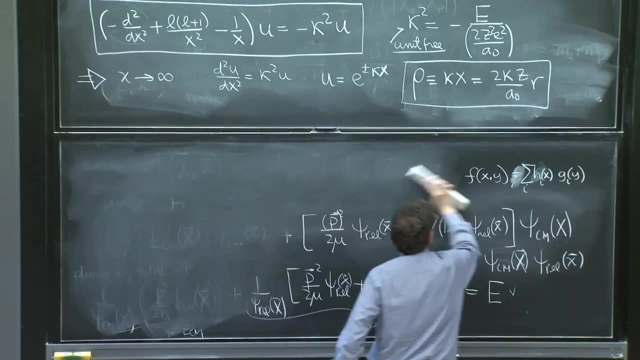 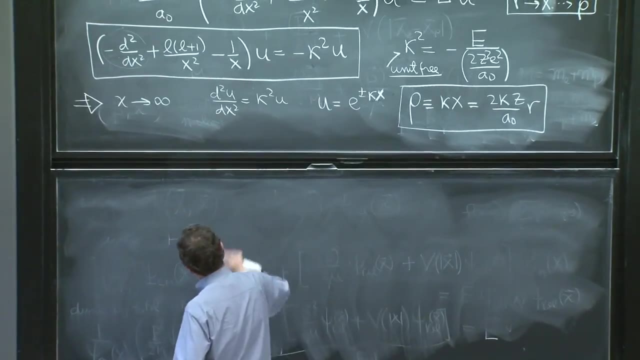 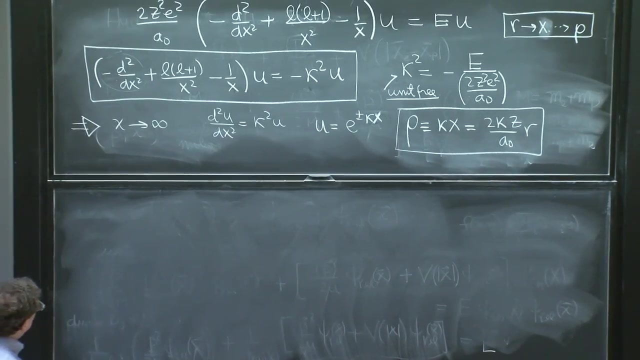 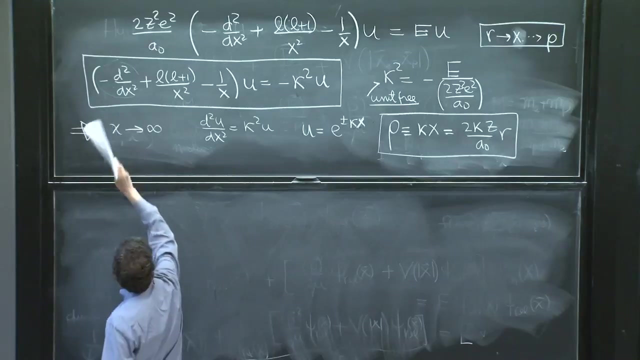 Well, It's going to be a little better. But in particular, the solutions may be a little better, But here it is. If you look at the differential equation here, think of moving the kappa squared. It's going to be 1 over kappa squared here below. 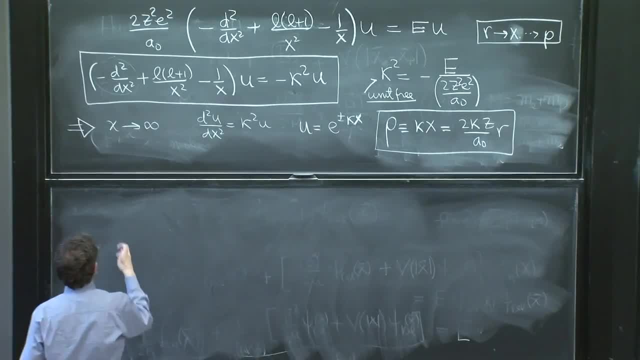 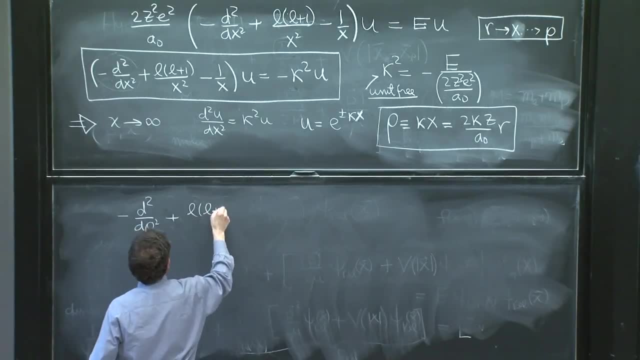 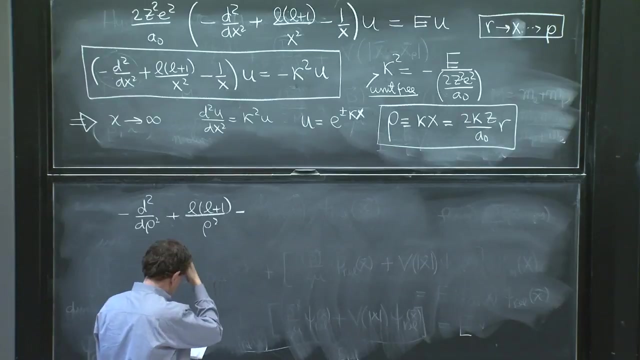 And then you see immediately it fits perfectly well in the first two terms. So you get minus d, second d rho squared plus l times l, plus 1 rho squared, And here it doesn't fit all that well. You would have 1 kappa left over. 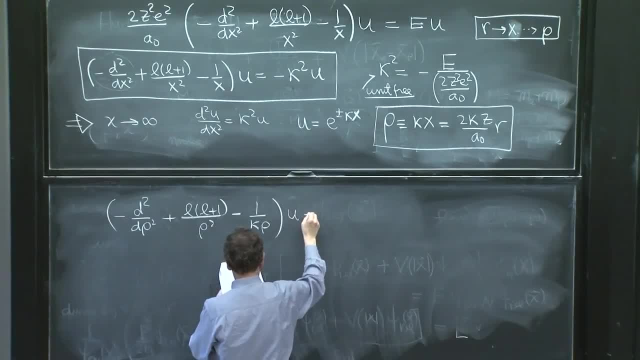 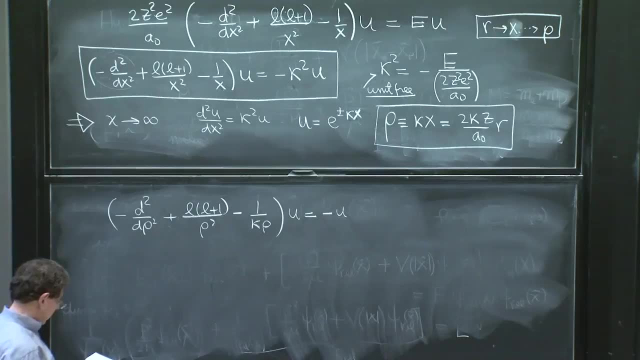 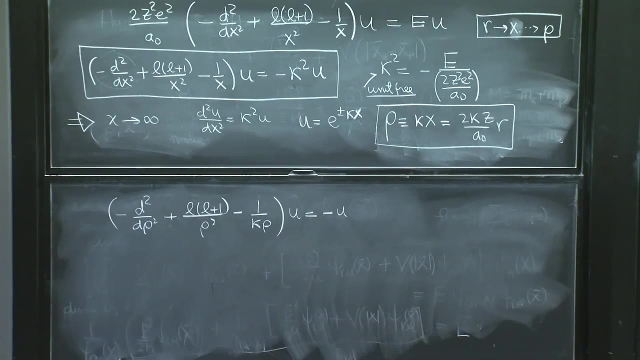 So 1 over kappa rho And you get minus u equals minus u. Yes, It's kind of suggestive. The kappa has almost disappeared from everywhere, But it better not disappear from everywhere. If it would have disappeared from everywhere, we would have been in problems because the equation would have: 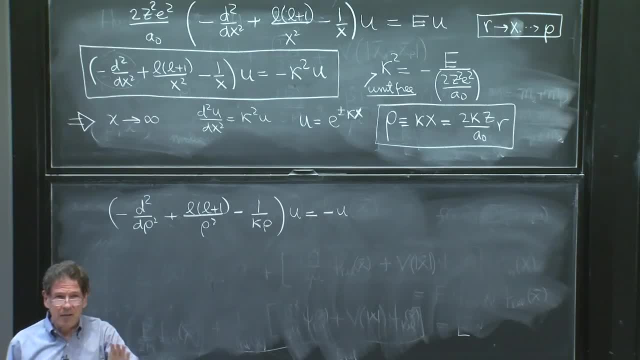 not fixed the energy. You see, we're hoping that the differential equation will have, as usual, solutions for some values of the energy and for the others not. So the energy better not disappear. It came close to disappearing, the kappa, But it's still here. 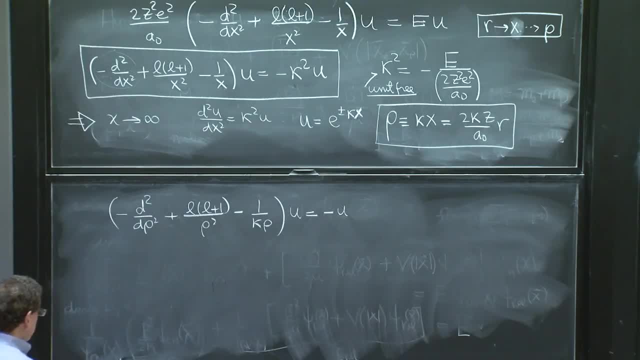 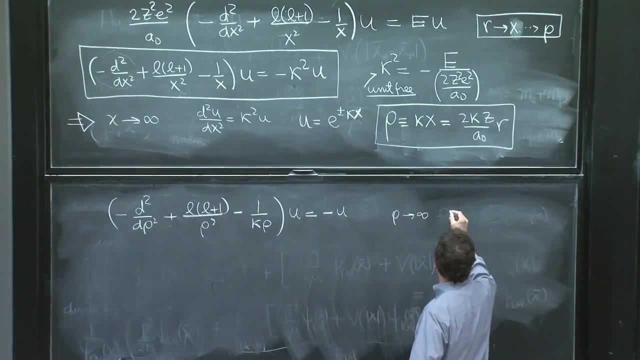 So we're still OK. And now you would say, OK, this is nice, This is nice. This is nice If you look at the right side. This is nice. So rho going to infinity. again, it works as we wanted. 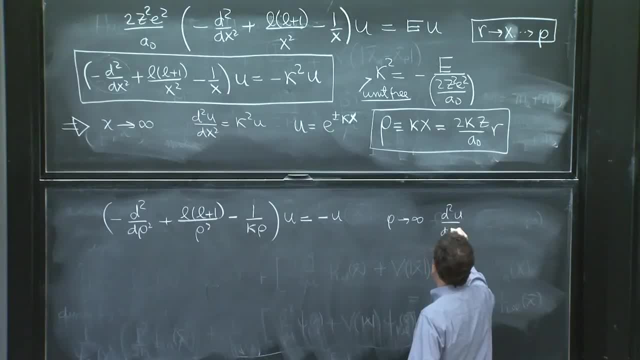 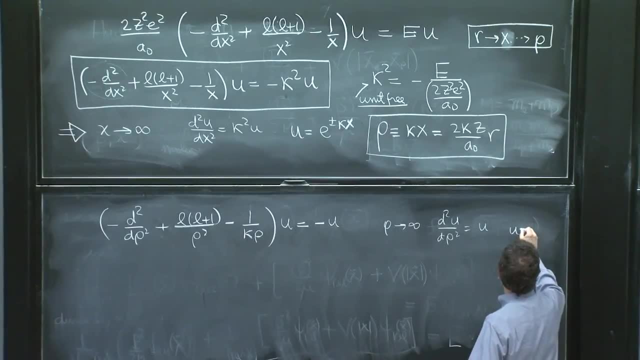 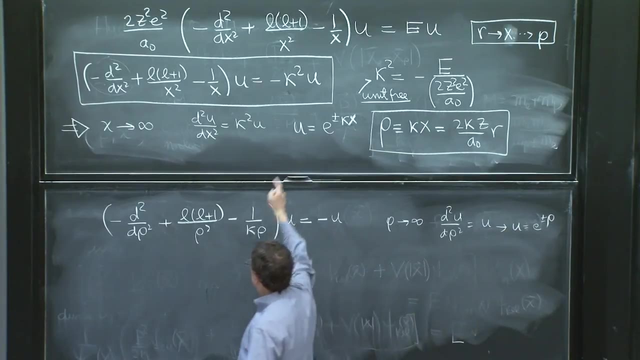 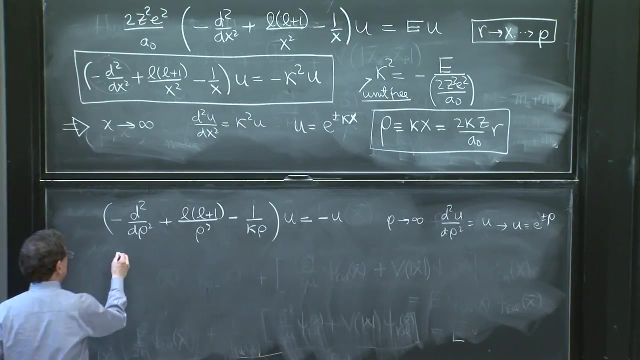 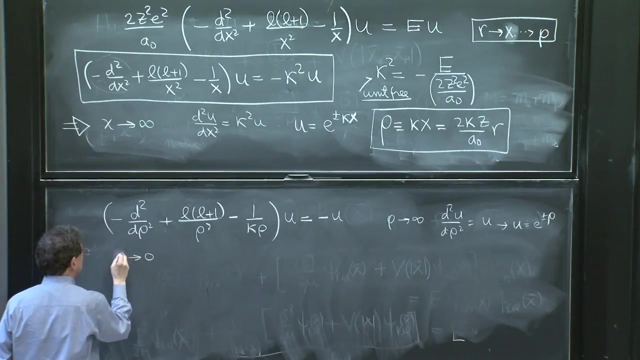 You get d second u d rho squared is equal to u And that means u goes to e, to the plus minus rho, which is what inspired this, And the other part of the solution is the solution at near r going to 0, or near x going to 0,, or near rho equal going to 0.. 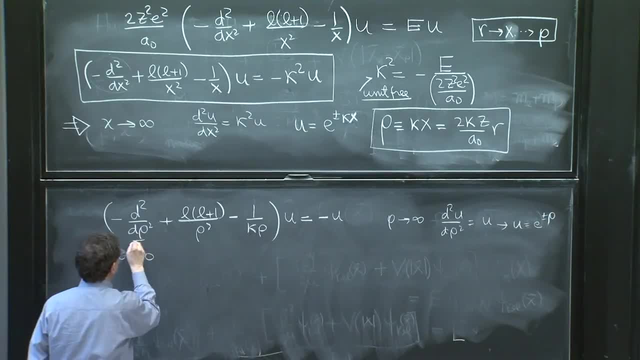 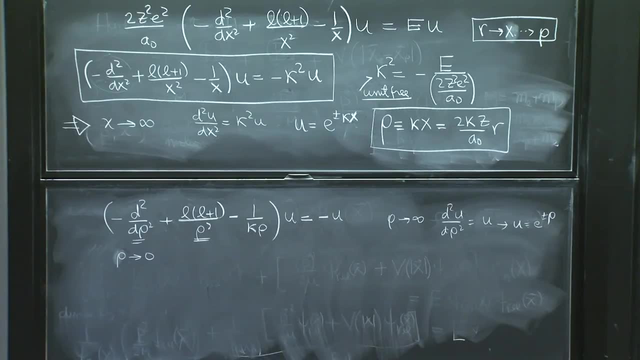 So near rho going to 0, you have these two terms And we actually did it last time. We analyzed what was going on with this equation last time, near rho equal to 0. And we found out that u must behave like rho. 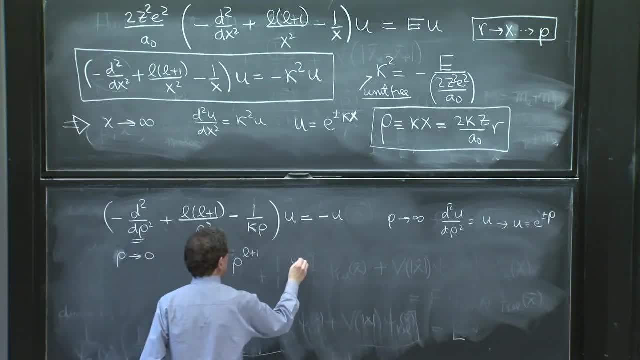 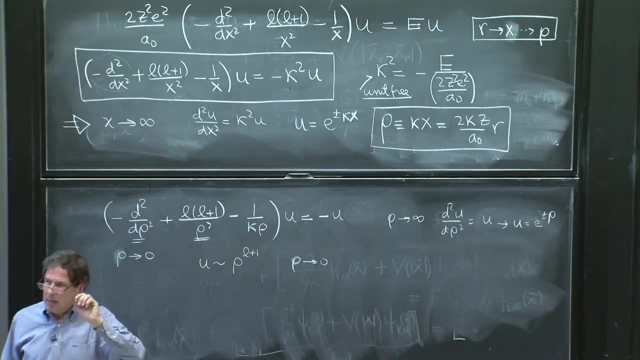 It must go to the l plus 1, for rho going to 0. So it was from these two terms the differential equation, And for rho going to 0,. remember the wave function must vanish, And how fast it should vanish. 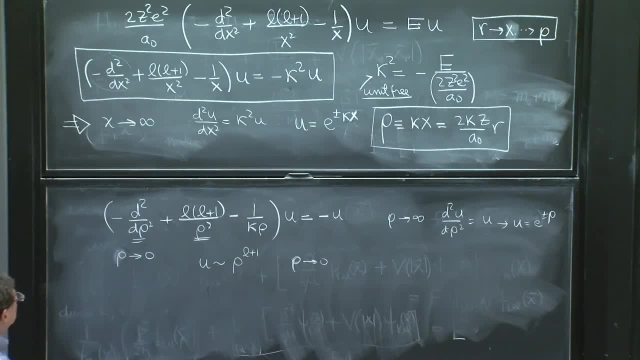 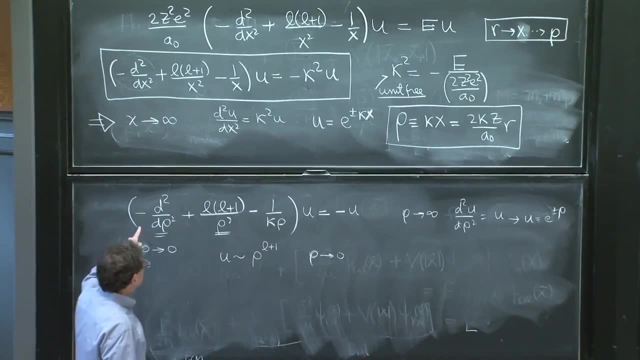 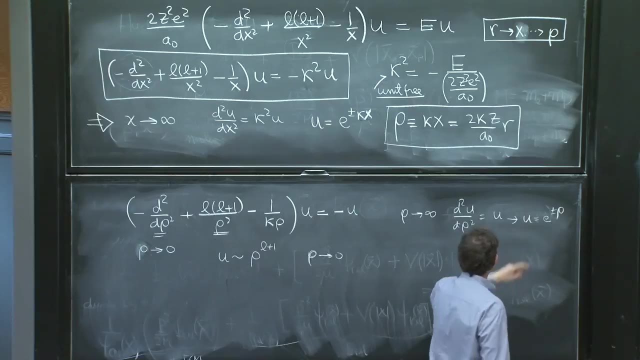 It should vanish to this power, to the l plus 1.. OK, So you know lots of things. OK, OK, So you know lots of functions. So, first of all, that this thing doesn't have necessarily polynomial solutions because it behaves exponentially. 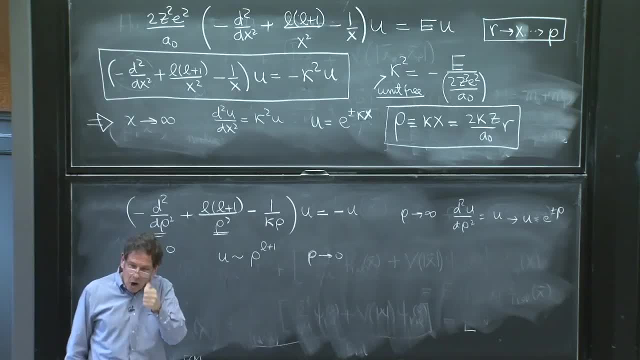 Moreover, you know it doesn't start with constant plus rho plus rho squared. It starts with rho to the l plus 1.. So it is pretty important to see all these things before you try to do a recursion relation, because recursion can lead you to funny things. 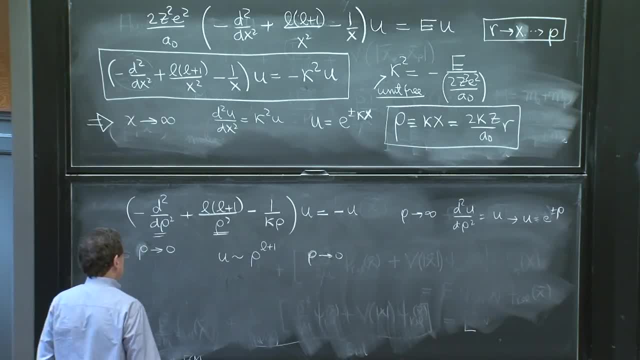 So here we go. What do we do based on all this? We try something better, which is we set u of rho the solution. We write an ansatz. It's going to be rho to the l plus 1.. That will have the right behavior for rho going to 0.. 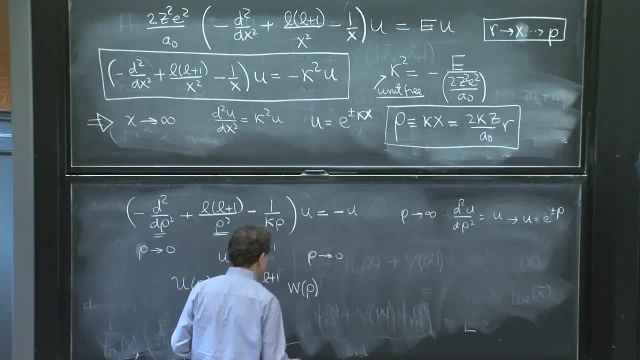 An unknown function. w of rho times e of rho, which is 0.. That's an unknown function. That's an unknown function. That's an unknown function. It's going to be e to the minus rho, which is the right behavior we want. 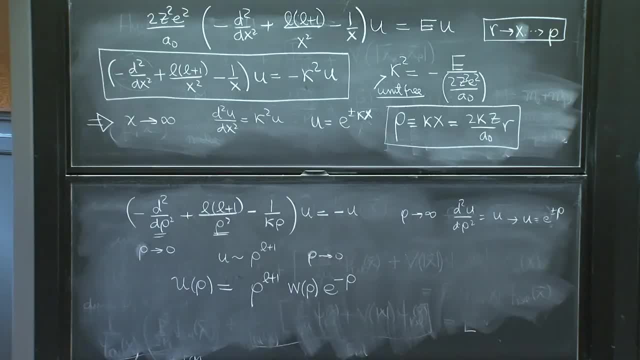 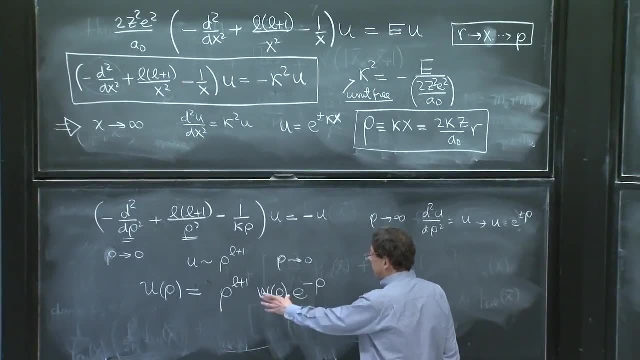 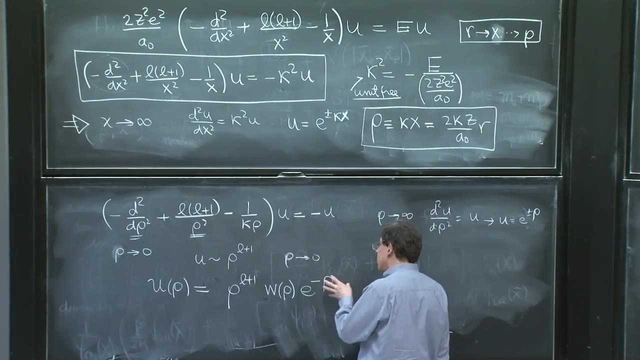 Now, there's no assumption whatsoever. when you write an ansatz of this form, You're just expressing your knowledge, because, at the end of the day, if omega or w here actually is undetermined, this w will have an e to the rho. that 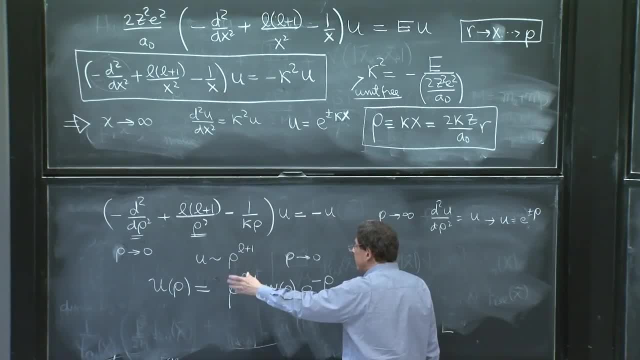 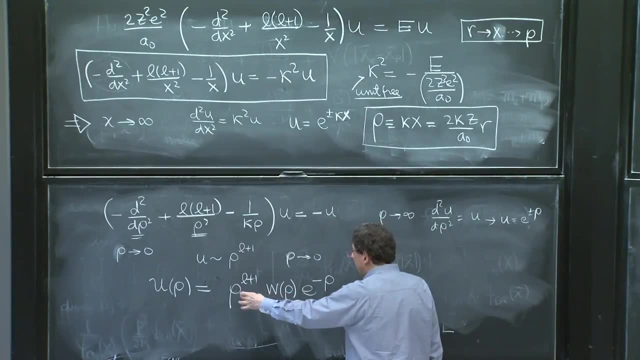 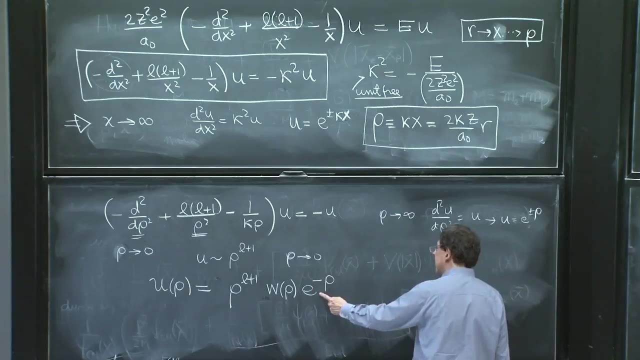 cancels this factor and maybe with some funny power that cancels this. This is just a hope that we're expressing that by writing the solution in this form. this quantity may be simple Because we know this is present in the solution for far large. 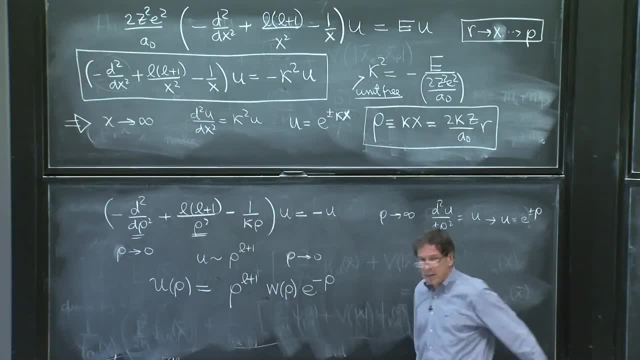 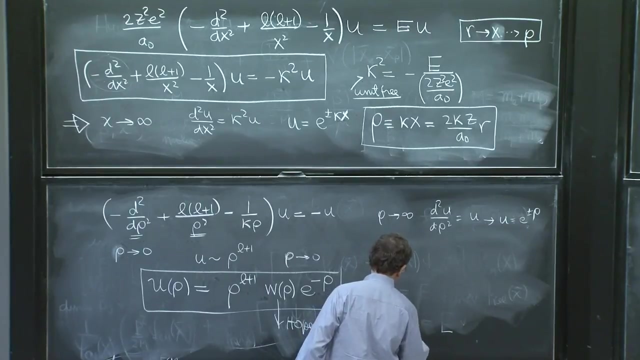 rho. This is present for small rho. Well, in between, we might have that. And when you write an ansatz of this form, you, You, You, You, You hope for a simple differential equation. 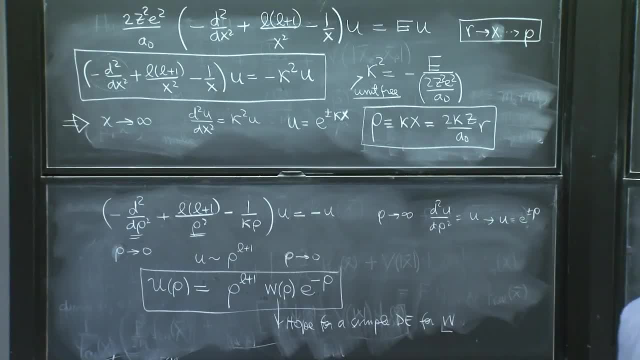 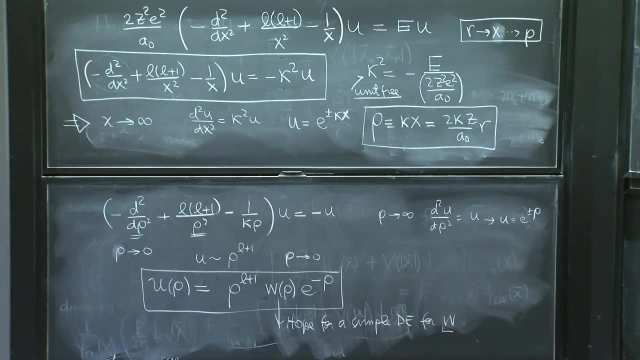 for w. So what do we get? Well, we can plug that ansatz into the differential equation that we already have And see what happens, And indeed that's what we'll do. I'll skip the calculation In my notes. it took me half a page. 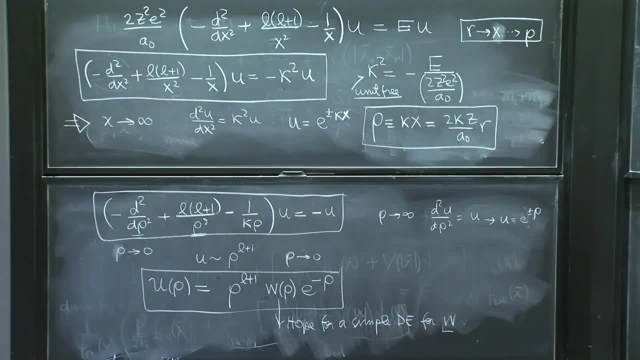 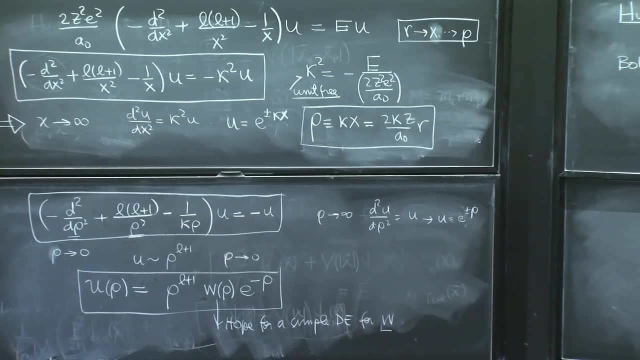 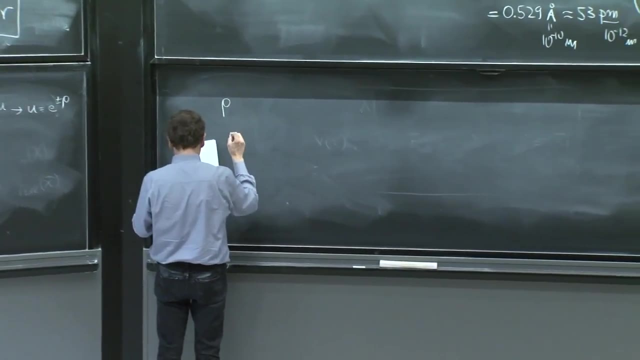 And I write big, So it's not too long. So what do we get? You get an equation that doesn't look that simple. I'm sorry, It just does. It doesn't look that simple, It looks like a step back, but it's not. 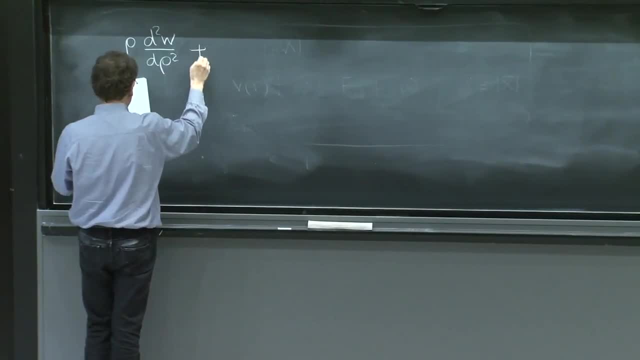 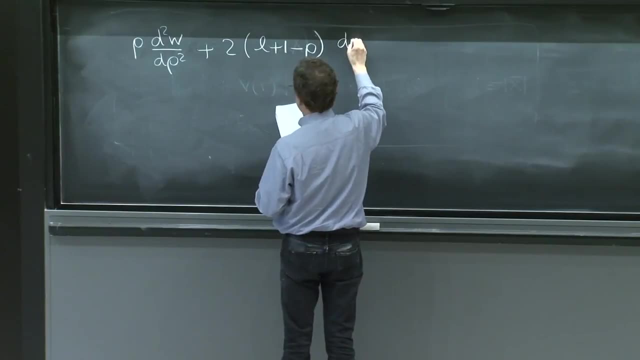 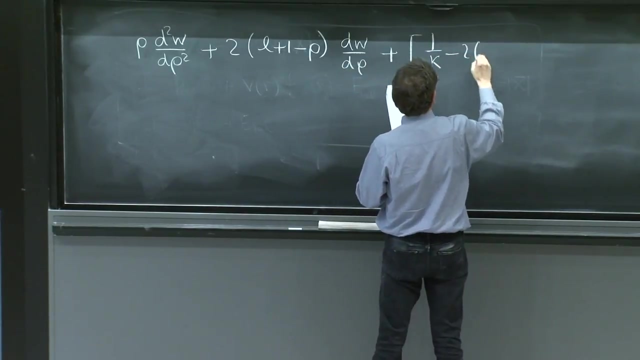 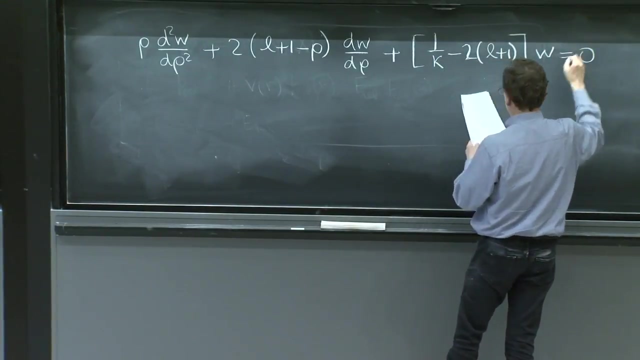 d second w d rho squared plus 2 times l plus 1 minus rho. Strange d w d rho plus 1 over kappa minus 2 times l plus 1 w equals 0.. d squared minus 1 over kappa plus 1 over kappa minus 1. 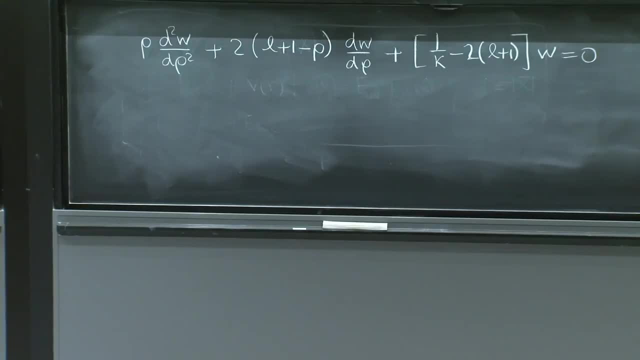 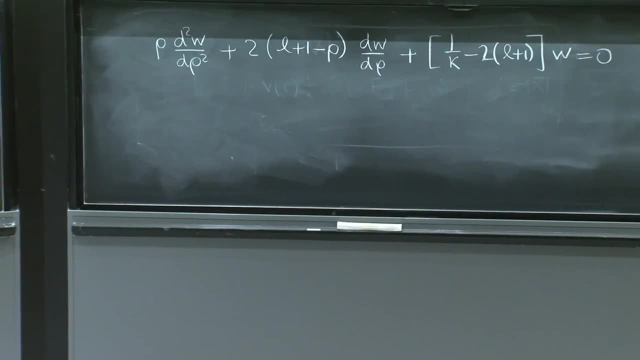 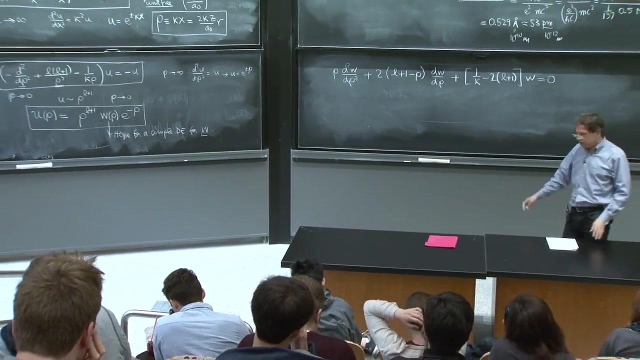 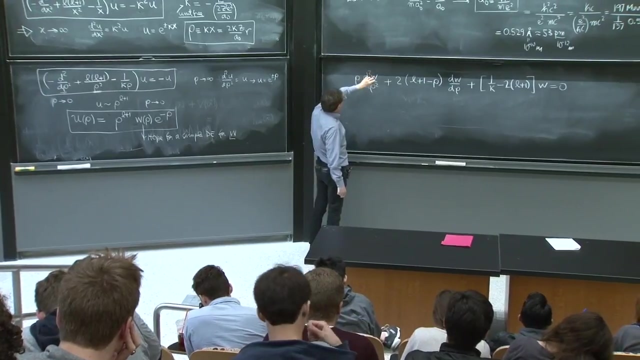 over kappa. OK, Aesthetically looks worse. Certainly that equation on the left board looked nicer, But actually it's pretty good, Because again now look at your recursion relation. How will it be If you take some power, fixed power? 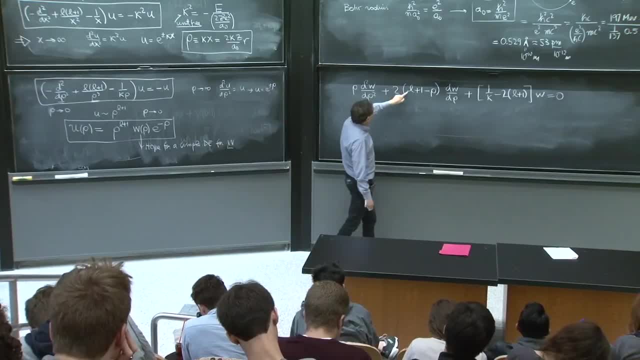 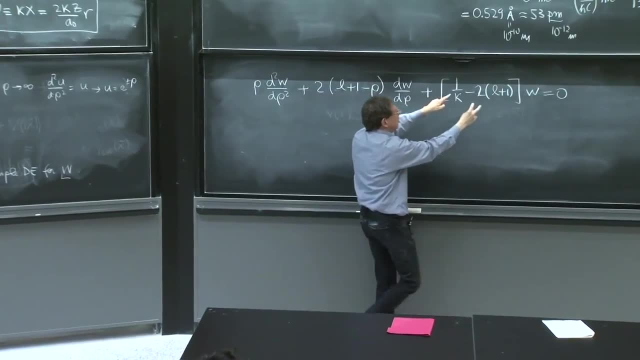 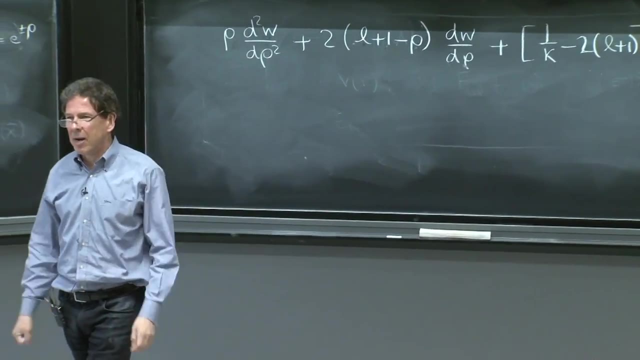 So here you lose one power. Here, with the l plus 1 on this, you lose one power. Here you lose nothing, And here you lose nothing. So you have either one power less or your power. So it's a one-step recursive relation without the gap.